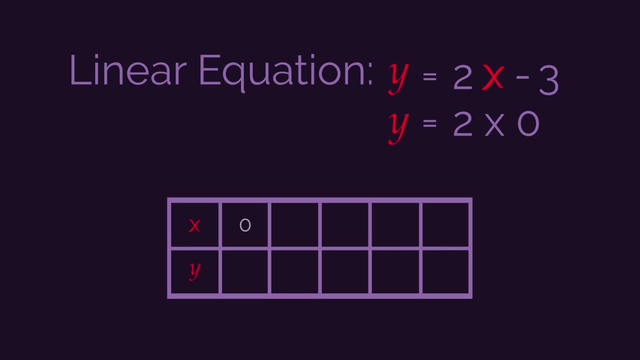 means y equals 2 multiplied by zero minus 3. So then y equals zero minus 3. So y equals negative 3. And we can enter this into our table: When x is zero, y is negative 3.. So now choose another value of x. Keep the numbers small, so let's go for x equals 1.. So then, 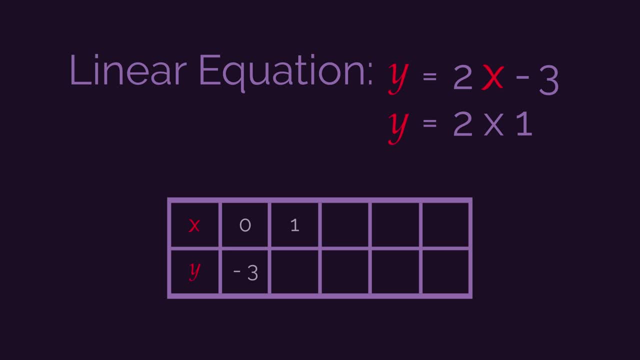 y equals 2 multiplied by 1 minus 3.. So y equals 2 minus 3, so y is negative 1.. And again we can enter this into our table: When x is 1, y is negative 1.. So now it's your turn. Work out the remaining three y values. 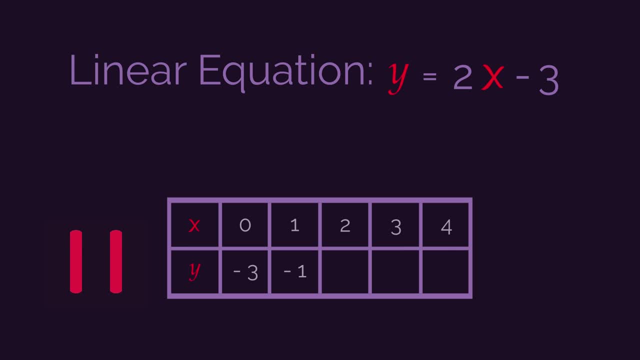 for the corresponding x values. Pause the video, work out the answer and click play. when you're ready to check, Did you get them right? 1, 3 and 5.. So we now have 5 sets of coordinates which we can. 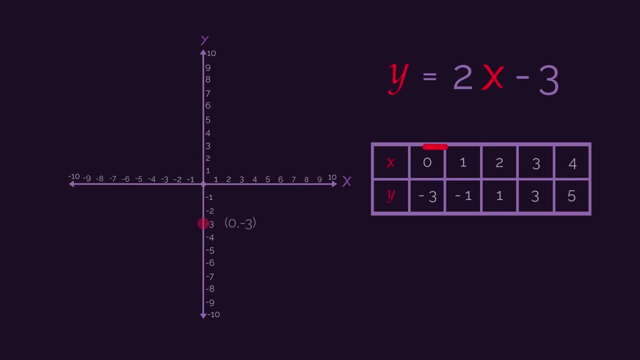 just plot onto our graph: 0, negative, 3, 1, negative, 1, 2, 1, 3, 3 and 4, 5.. So now we just need to join up our coordinates with a straight line using a ruler. Make sure. 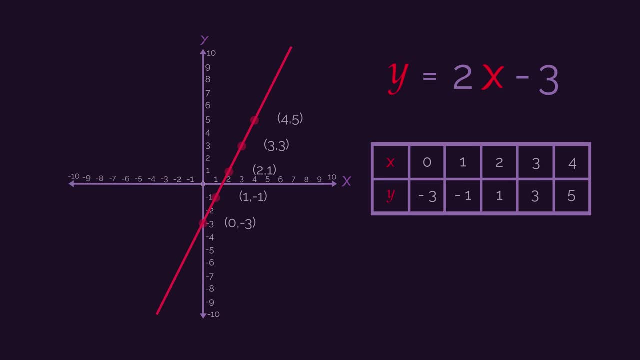 you extend the line the whole way across the graph and label it with its equation. Simple: We plotted 5 coordinates, but as a rule you need a minimum of 3 coordinates to accurately plot a straight line. We just had an extra 2 in case we made a mistake. 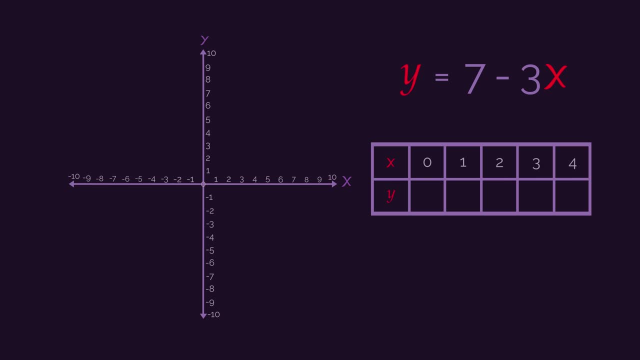